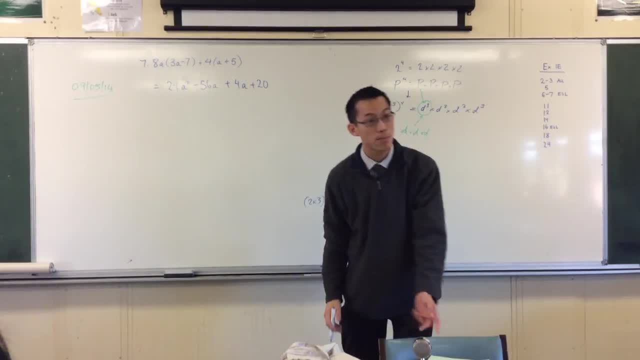 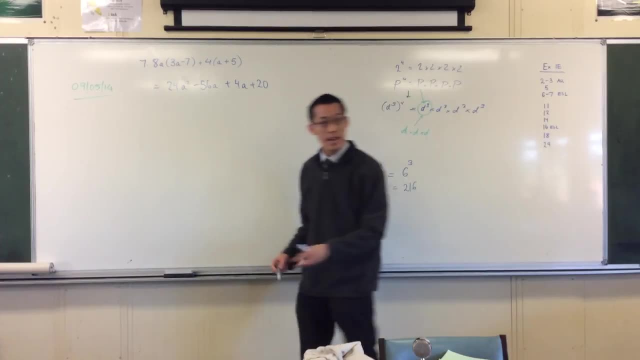 Now I've done my expansion. Then they say expand and simplify. So you have a look and you see, are there any like terms? Where's my green arrows? And the answer is yes, there are some like terms. There's a's here and there's a's here, okay.